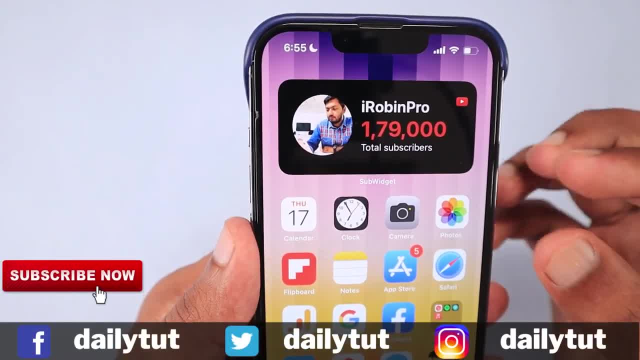 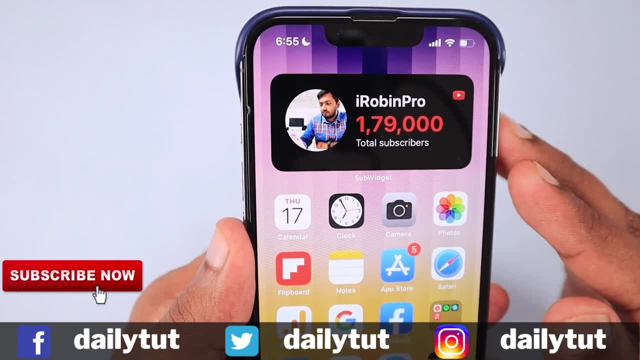 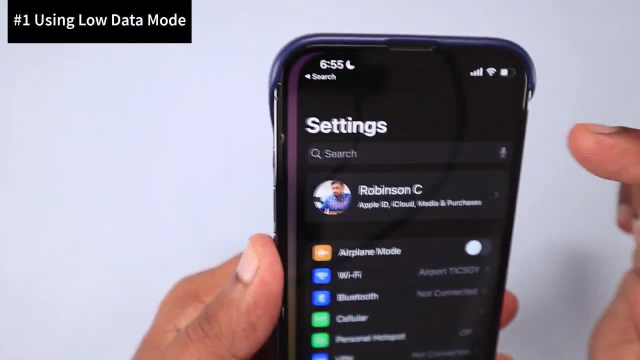 limit. In such cases, you might be wondering like: what is the reason behind it? and you may not be able to figure it out initially. which application or which services are consuming your data without your knowledge? So the first troubleshooting step that you need to check is go to settings and then 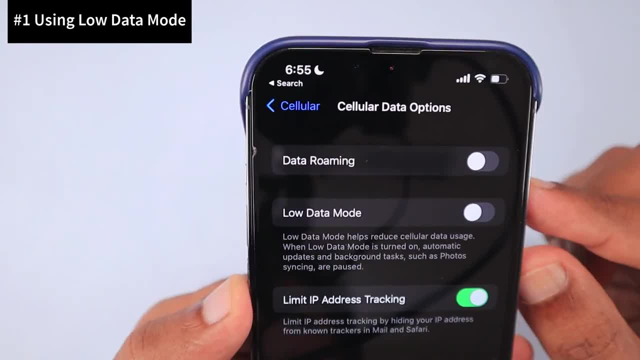 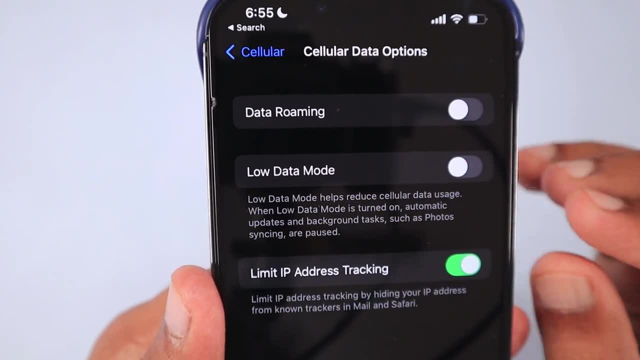 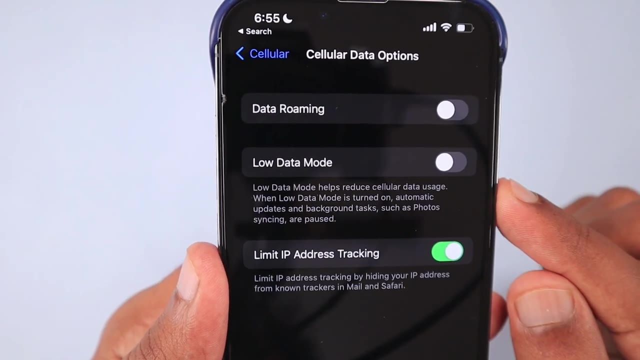 navigate to cellular and here you can see cellular data options, And if you're not sure about which application or service is actually consuming more data without your knowledge, then you can turn on the low data mode. This is kind of a basic troubleshooting step, and it is not a perfect solution- is what I believe, because it is important to figure out which. 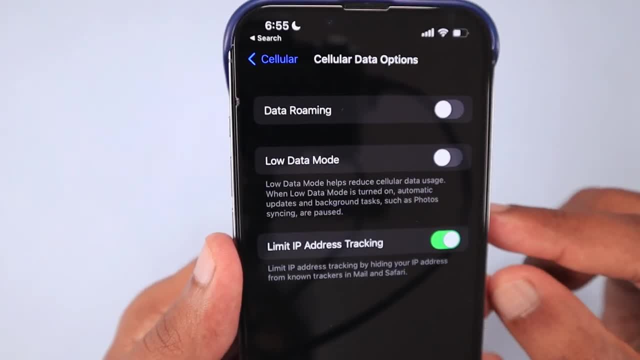 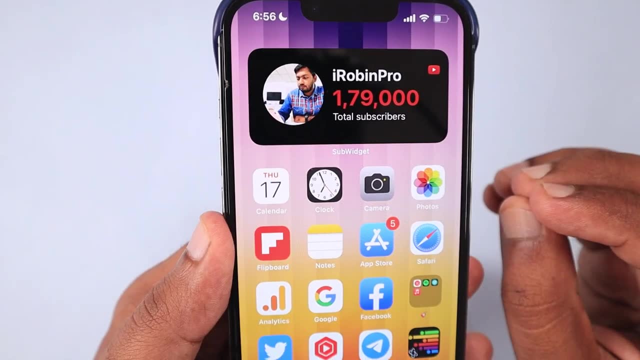 application is actually using it. We will see in the upcoming possible steps. Data consumption for the third-party apps are very much restricted, So the possibilities of third-party applications like Facebook, YouTube or any other application are very much restricted. So the possibilities of 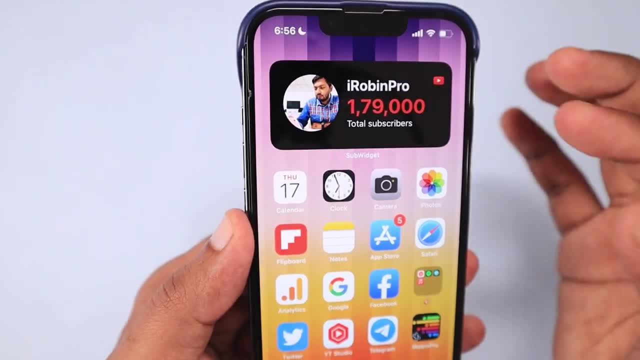 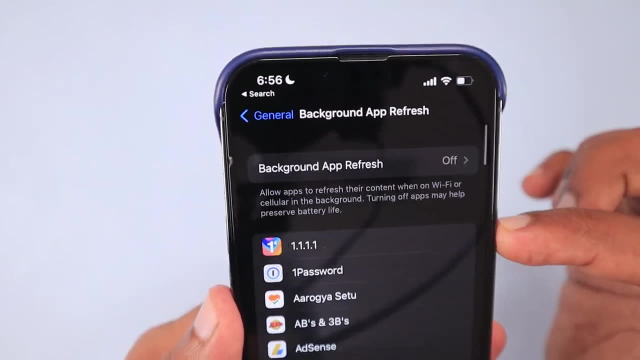 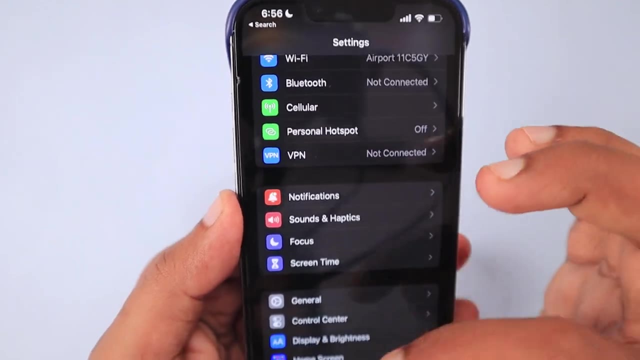 using your data in the background is very less. Some users suggest to turn off the background app refresh from settings general and background app refresh. I'm not sure how effective that is going to be. As I said before, it is important to pinpoint where the problem is, The next important. 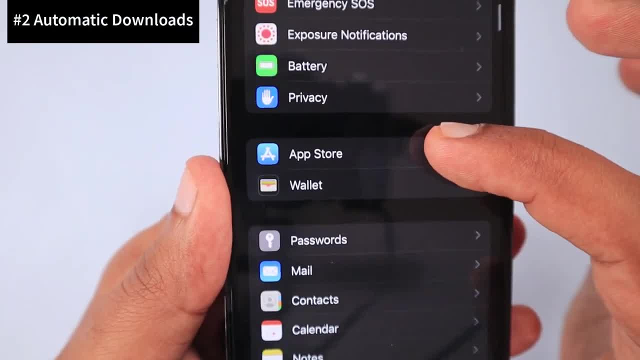 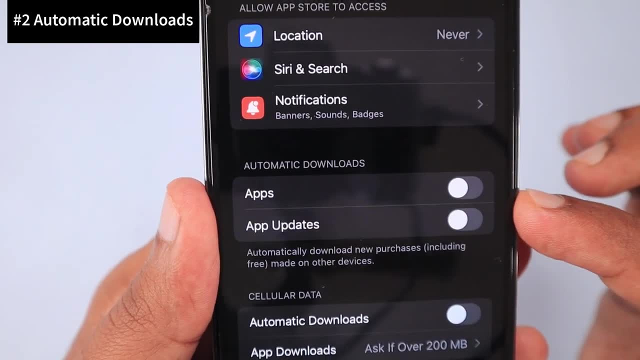 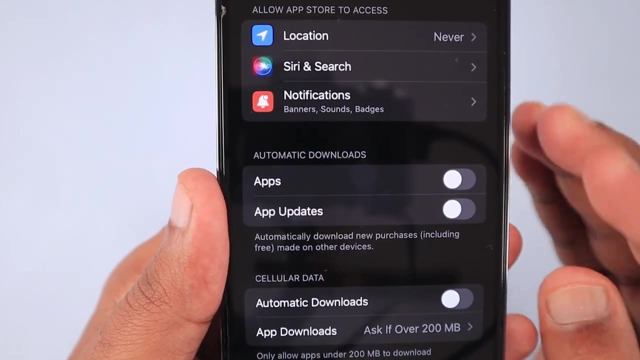 step that we must do is, in the settings page, scroll to the app store section and navigate inside the app store settings and there you can see the automatic downloads option. If you have recently reinstalled your iOS, performed an iOS restore, or you have bought the iPhone or iPad, 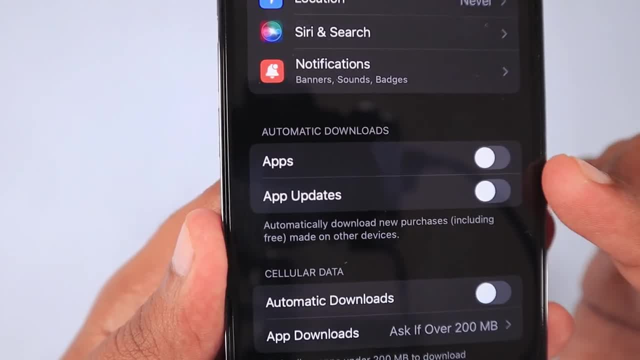 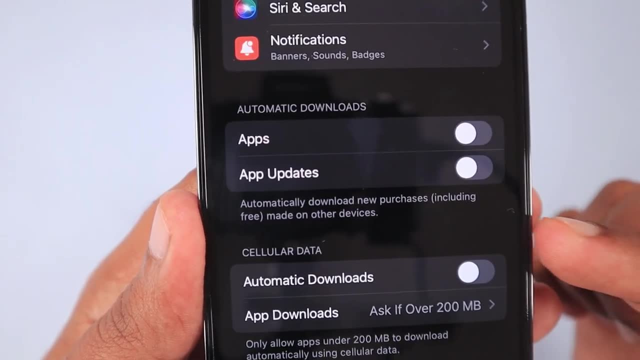 recently and you are using it for the first time, by default, these settings could be turned on. So if you are not sure which application or automatic updates or any other system related services are using the data in the background, you can turn off these toggles. The automatic downloads for. 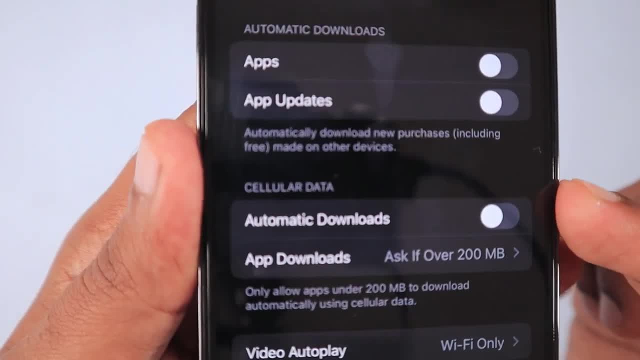 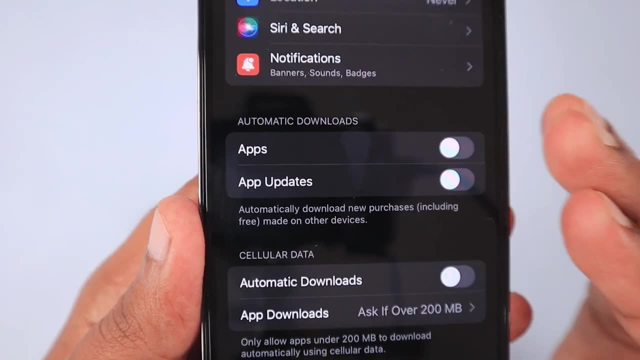 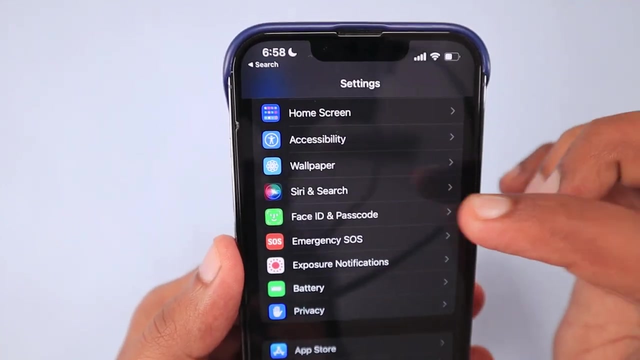 the applications for the app updates, and especially the cellular data section, gives you the option to turn off the automatic downloads in general. So you can turn off these to prevent any applications updating or even system software related updates happening through the cellular data in the background. And the next important troubleshooting step is go back to settings and then navigate to. 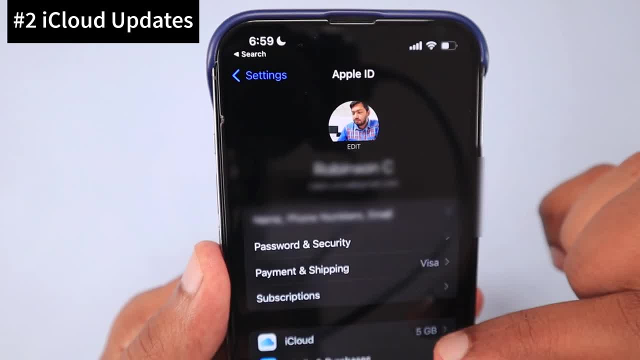 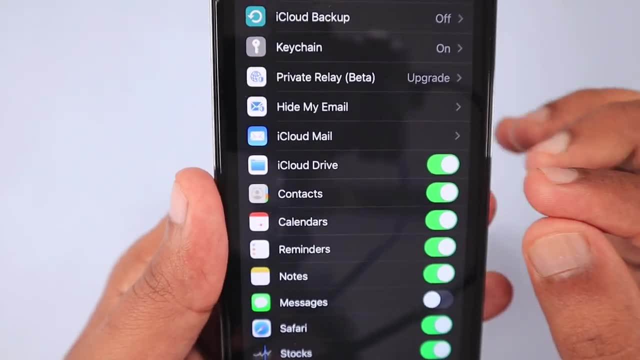 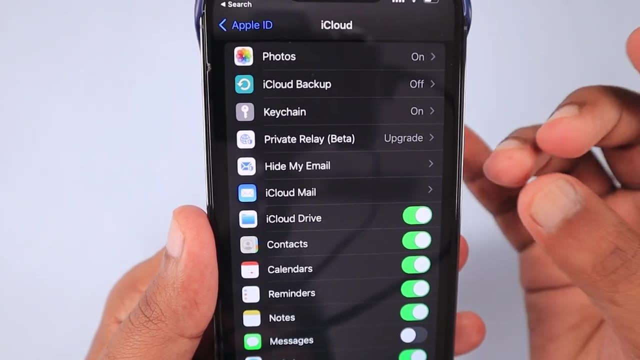 your iCloud profile section and then navigate to iCloud. Here you can see iCloud, So navigate inside and here you will see all the iCloud services that are allowed to use the network, especially if you have reinstalled the OS or you know you have bought the iPhone or iPad. 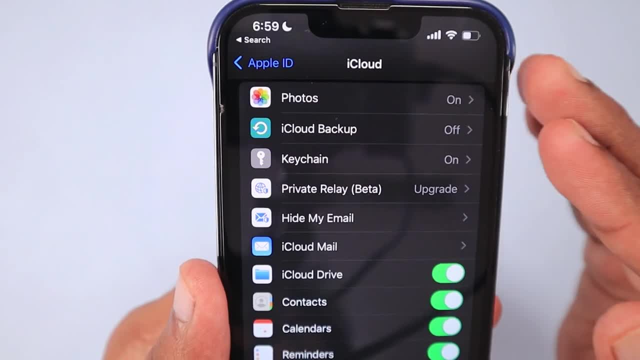 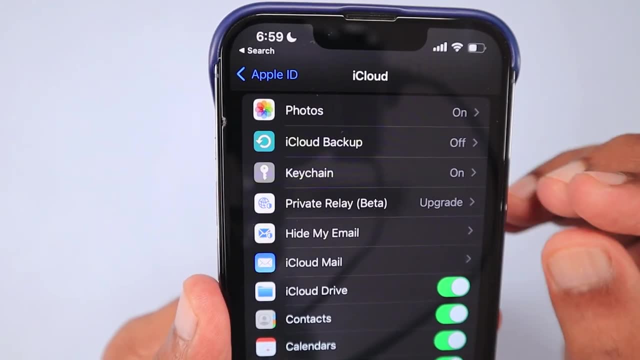 cellular model recently. Most of the time when you sign into your Apple account after creating it for the first time, these features you know could be turned on by default. So, without your knowledge, the iCloud services could be using the data in the background and gives you a surprise in. 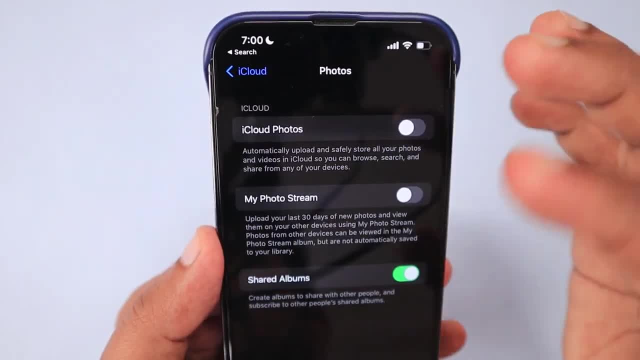 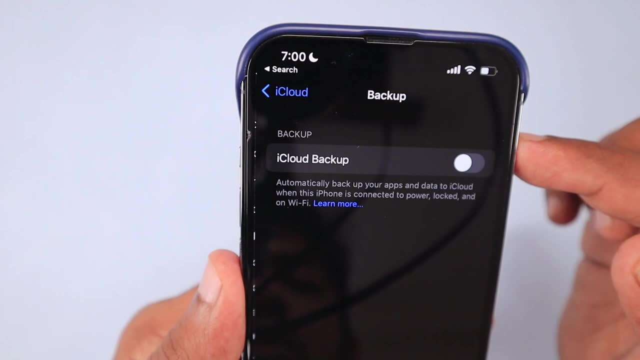 the morning that all your photos and videos that you have shot before you know like in the past few weeks, all of a sudden started to upload to your iCloud account, to your iCloud photos. So this is Wi-Fi, as far as I have understood. it doesn't use your mobile data for performing the iCloud. 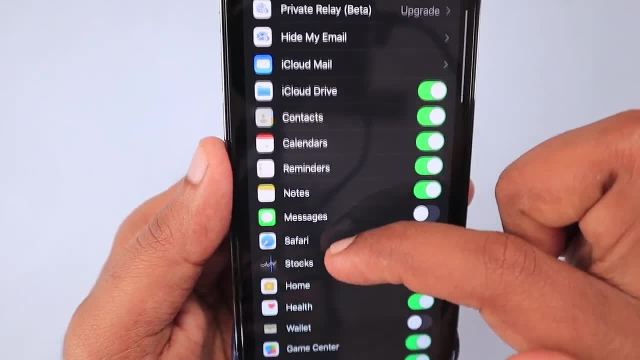 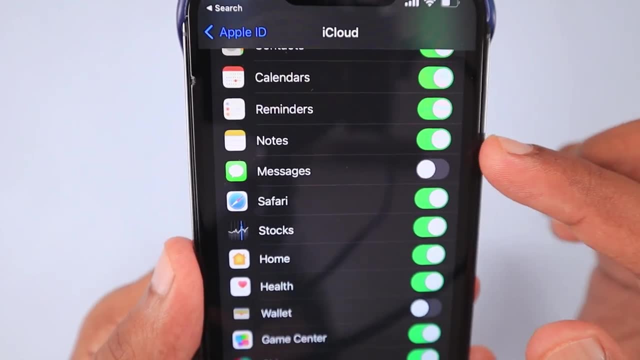 backup, but still you can manage and control it. And the next important thing is: all these services are not going to consume more data to keep itself up to date. For example, your calendars, your notes, all these things are very important, So don't turn off these things without understanding. 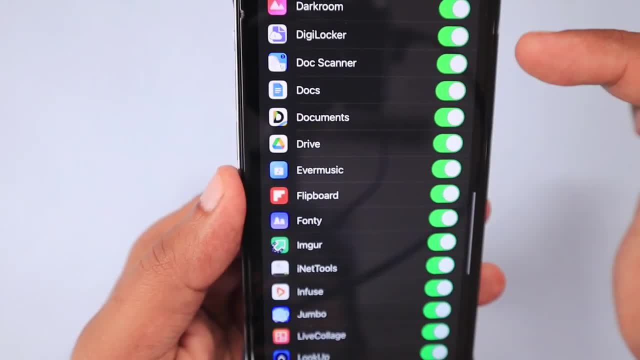 what each of the service is for. But below that you can see all these applications. you know if you are downloading anything or recently downloaded anything to any file manager applications, So you can see all these applications. So you can see all these applications. you know if you are downloading anything or recently downloaded anything to any file manager applications. 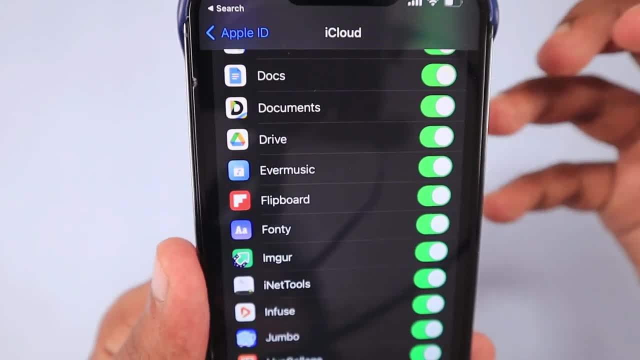 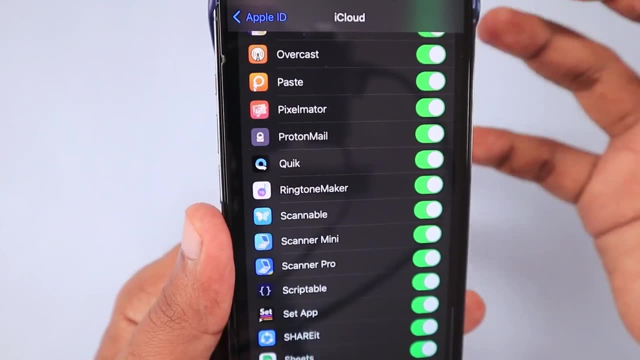 like documents or any other application, and the sync operation happens in the background. if it uses the mobile data, then possibly it could consume more data over the night and it may surprise you in the morning with the data. daily limit has already been exhausted, So take control. 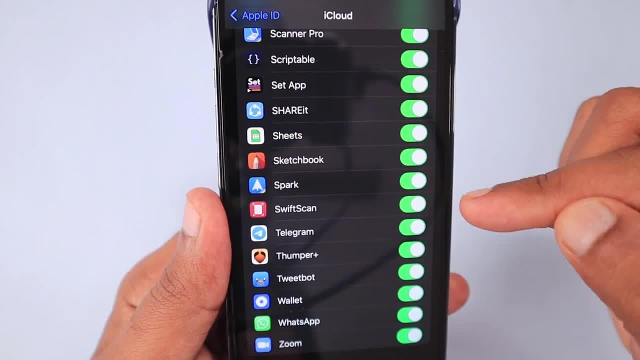 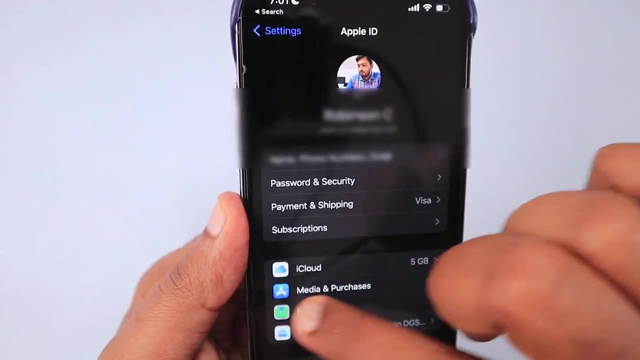 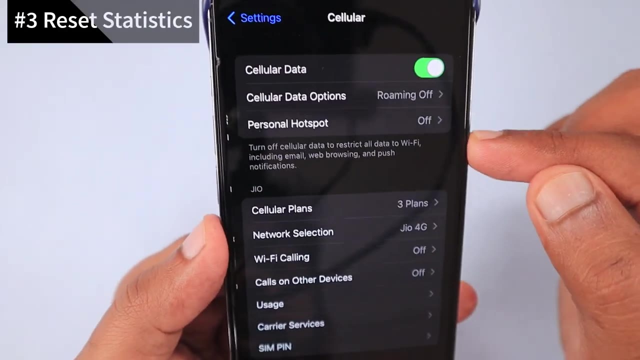 of these applications decide which iCloud services the application should use your iCloud account, iCloud storage and service in the background. So that is important. you can turn on and turn off any application that you don't want the cellular data to be accessed with, And the next important thing is to navigate back to settings and then cellular scroll to the bottom. 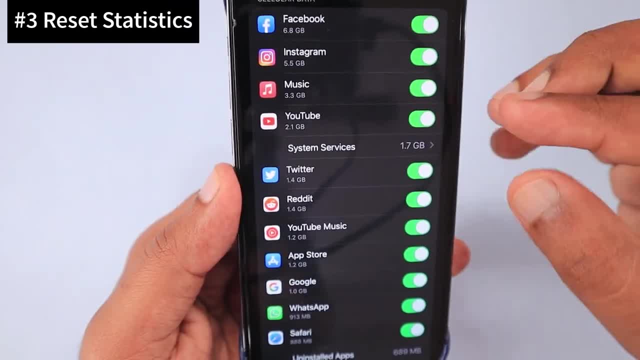 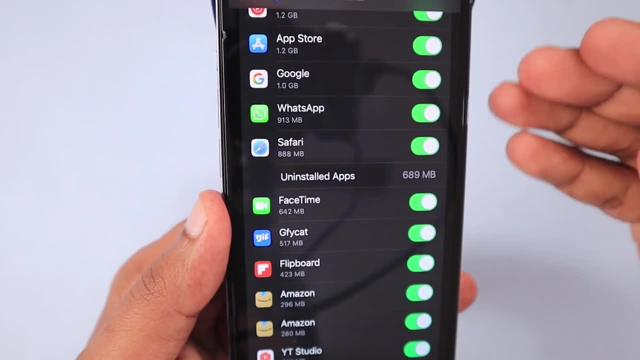 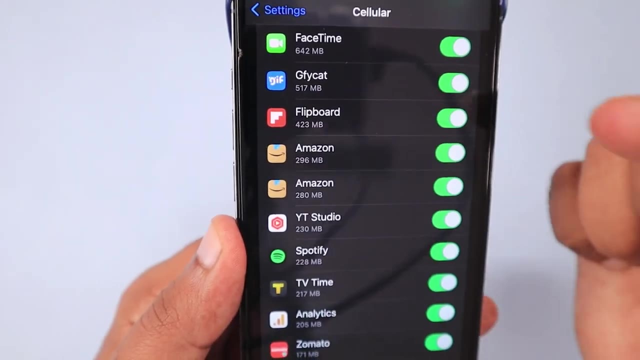 here you can see the statistics of all the applications that you have installed in your iPhone, even the system services and any uninstalled apps that have consumed. you know recently if you have removed any application. Still it stores all the details about the applications that consumes. that allows to use the mobile data in general.